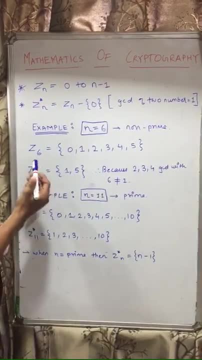 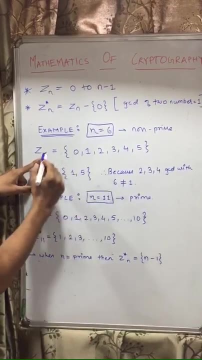 that GCD of two numbers should be equal to one, likewise if 6 and 0. so we have to exclude 0 from it. and now we between two number, 6 and 1. so GCD of 6 and 1 is 1. so 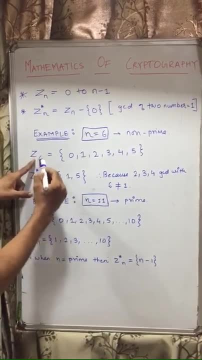 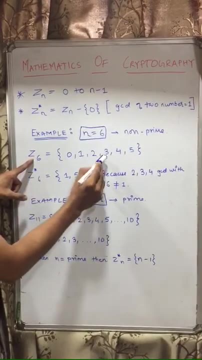 will include in Z star 6. 1 now will go to 6 and 2, the GCD is 2, so will not include the Z star set now 6 and 3, the GCD is 3, so still will not include that in our Z. 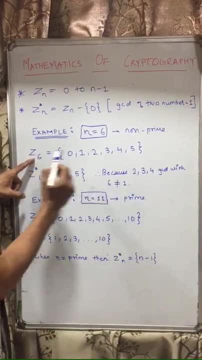 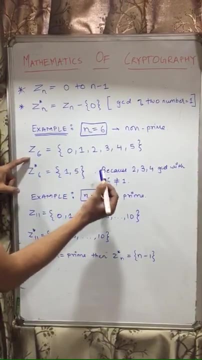 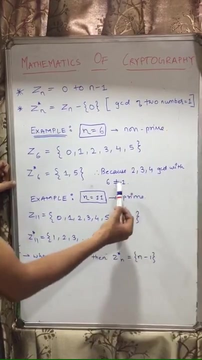 star set. now Z, 6, 6 and 4. so GCD is 2, so it will also be not include now 6 and 5 that GCD is 1, so it will be included in a set. so because 2, 3, 4, GCD with 6 is not, 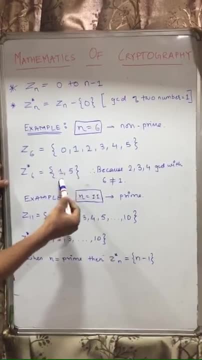 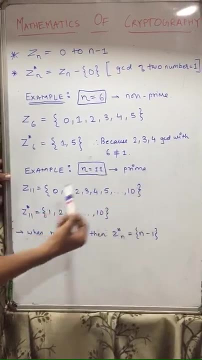 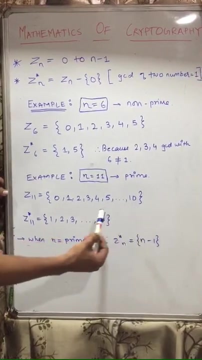 equal to 1, so will not include in Z star 6 set. okay, now another example. this was a non prime, now it will be prime. so when n is equal to 11, so it is a prime number, so that Z 11 will be equal to 0, 1, 2, 3, 4, 5 till 10 and Z star 11 will be the. 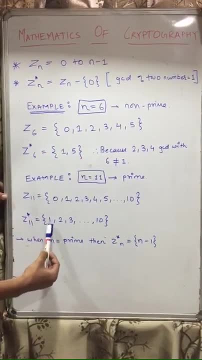 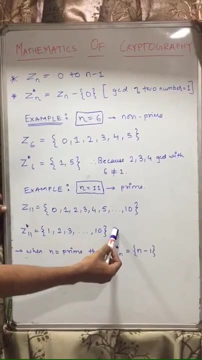 GCD of two numbers, as I said. so 11 and 1 GCD will be equal to 1, as 11 is a prime number. so all the numbers except 11, all the numbers except 11, will be included in the Z star section. so 1, 2, 3. 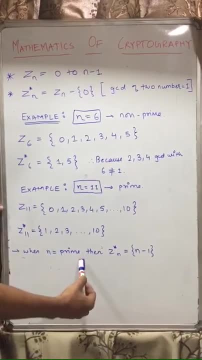 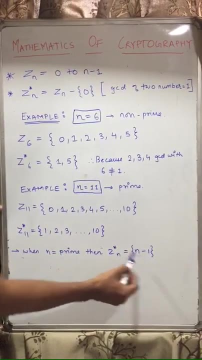 4 till 10. so when n is prime number, then Z star n will be equal to n minus 1. so n is 11. so minus 1, 10, so 1, 2, 3 till 10. so all the numbers from 1 to 10 will be. including Z star 11. thank you guys.